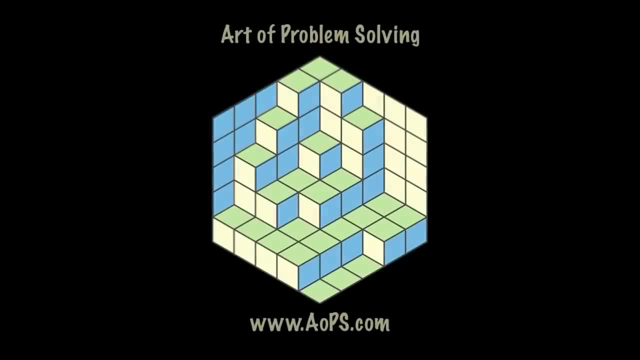 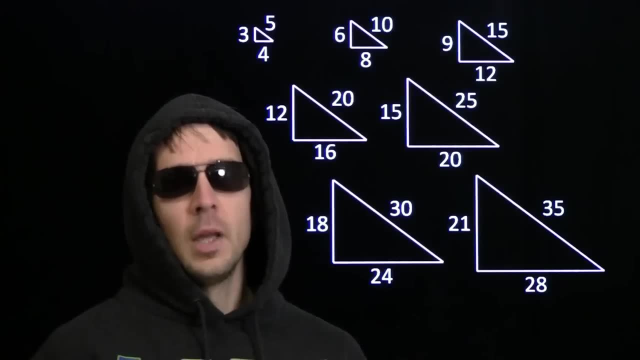 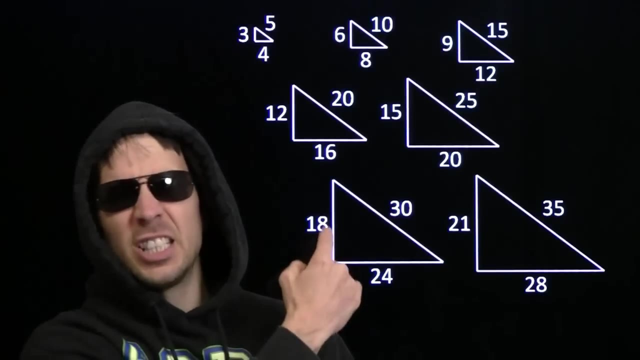 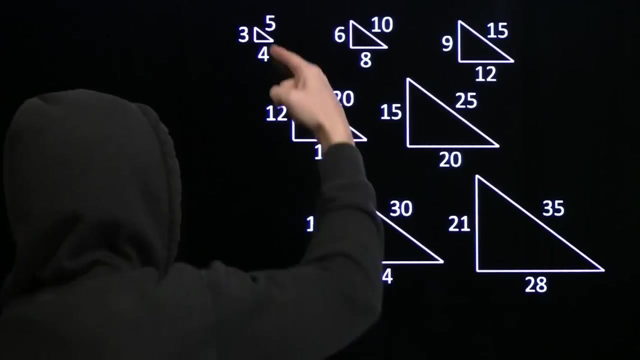 All right. other guy, You challenged me to go find a bunch more right triangles in which all the side lengths are integers. Check it out. Look at all the ones I found We got: 3 squared is 9,, 4 squared is 16, 9 and 16 is 25.. That's 5 squared 6 squared 36.. 8. 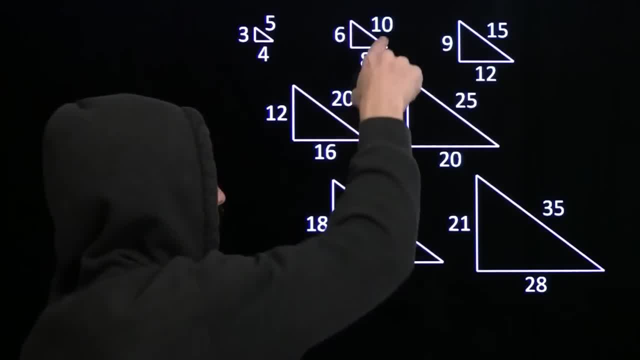 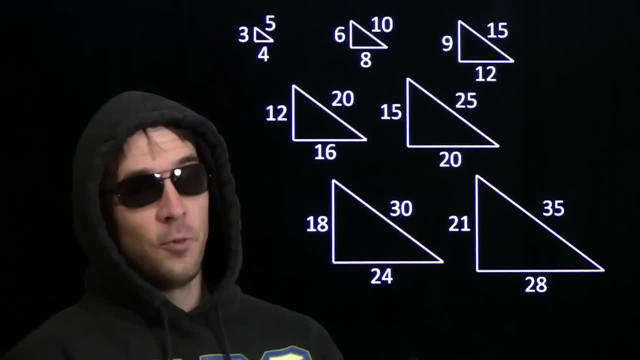 squared is 64.. 36 and 64 is 100.. That's 10 squared. Wanna jump down a little lower? Let's try that: 15 squared is 225.. 20 squared is 400.. 225 and 400 is 625.. That's 25 squared. 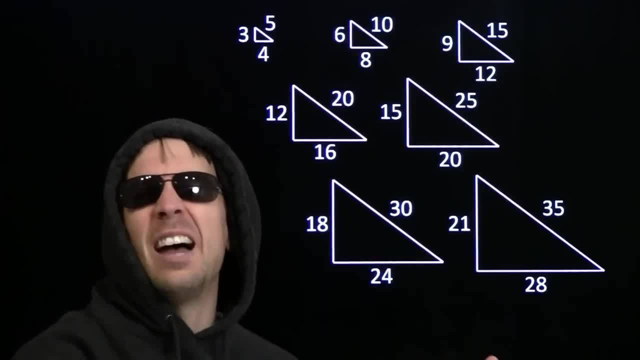 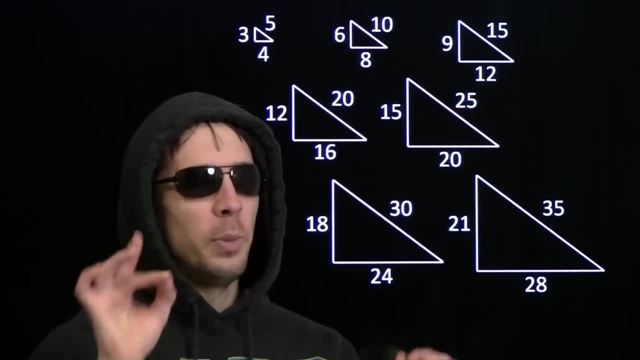 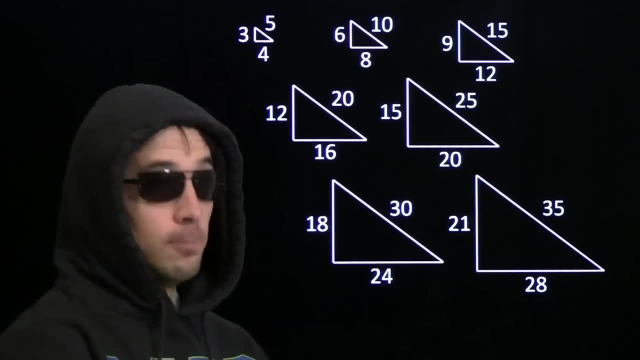 That's right. I can go on and on and on like this. I can go on forever. I can find all the right triangles with integer side lengths that you want. I found a really cool pattern. Check this out. We got 3, 4, 5.. We got 3 times 2, 4 times 2, 5 times 2.. 3 times 3, 4 times 3, 5 times. 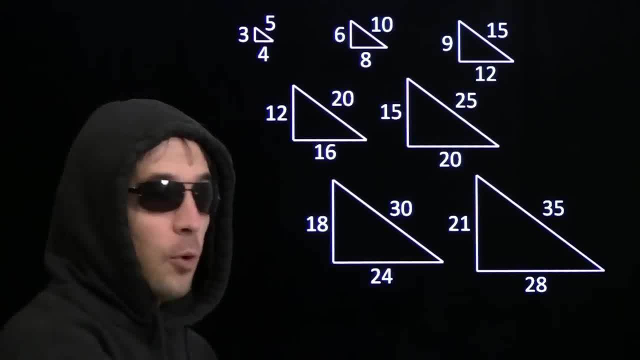 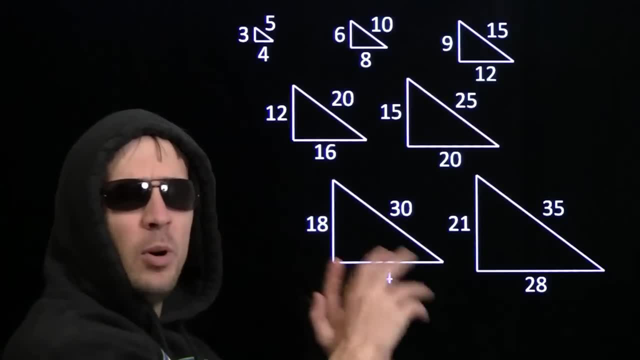 3.. 3 times 4,, 4 times 4,, 5 times 4.. And we just go on and on and on like that. Right here we got 3 times 7,, 4 times 7,, 5 times 7.. We just keep on going. I can multiply 3,. 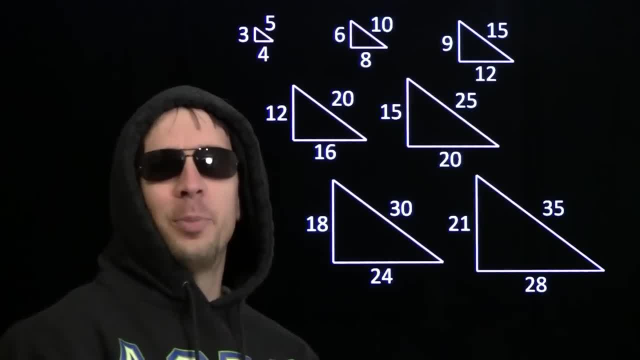 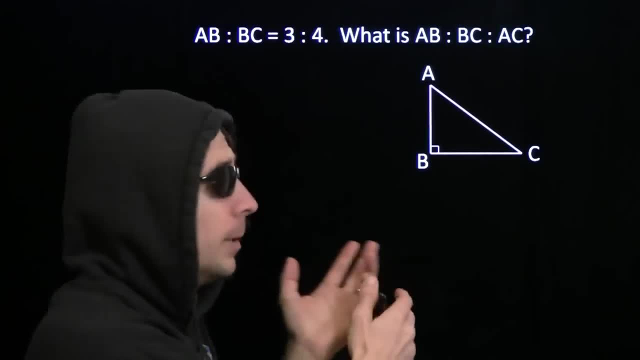 4, and 5. by anything I want to You, don't buy it. Check this out. I can even prove it to you. Alright, so we got a right triangle. Now I'm just going to tell you and say, hey, the legs. 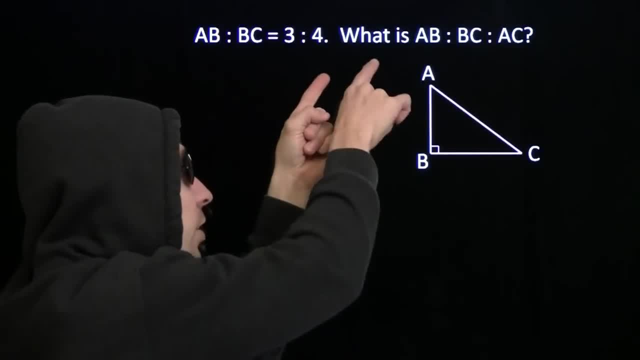 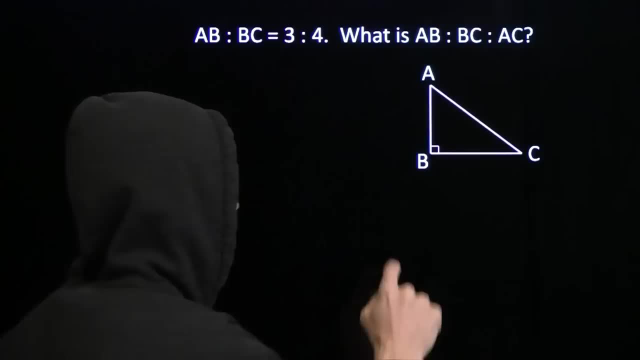 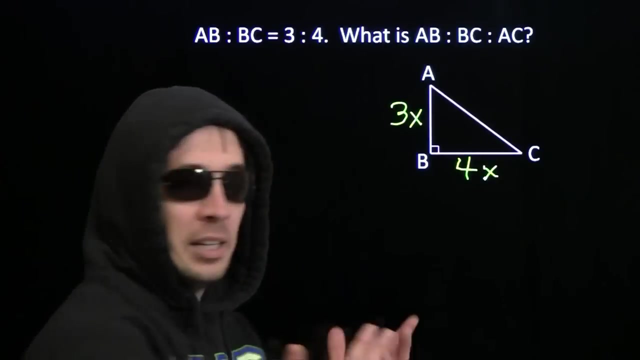 are in the ratio 3 to 4.. That's it, And I'm going to find the ratio of all three sides. So what this means? the ratio of the legs is 3 to 4.. That means that for some value of x, this leg is 3x, this leg is 4x. Now I've got a right triangle. I've got two of. 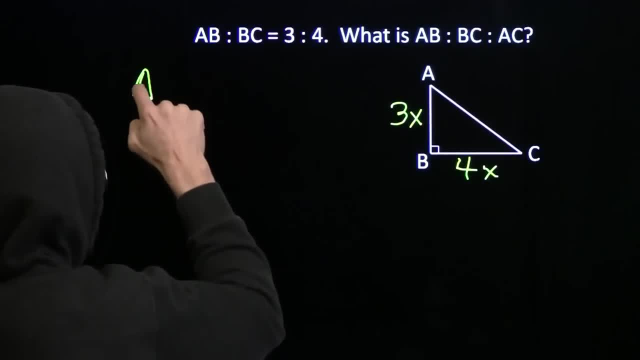 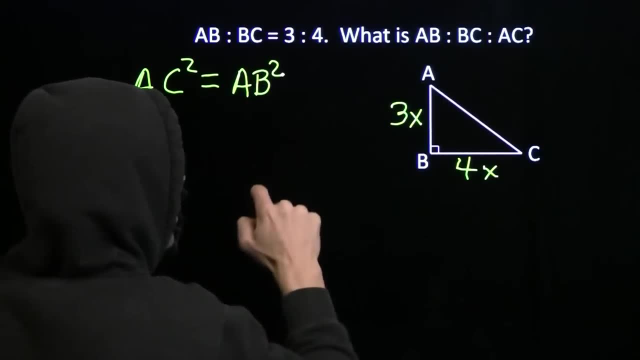 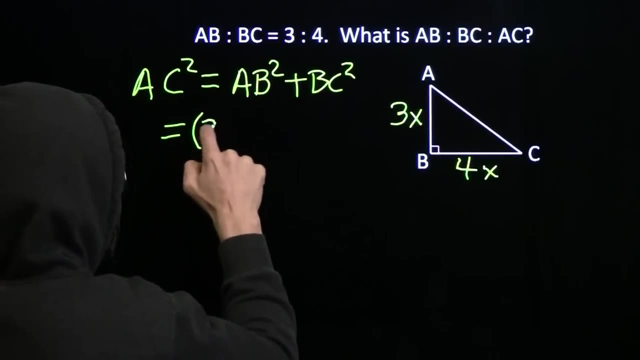 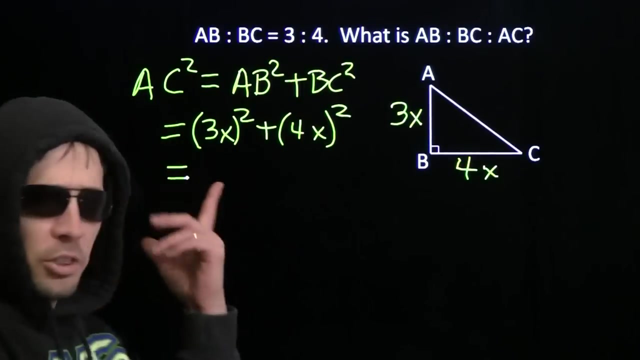 the side lengths. I can break out the Pythagorean Theorem. Alright, AC squared equals AB squared plus BC squared. And now I just substitute these in. This is going to be the square of 3x plus the square of 4x. Now we square the 3x, we 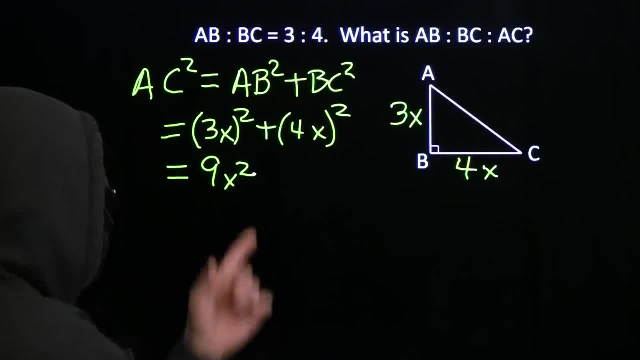 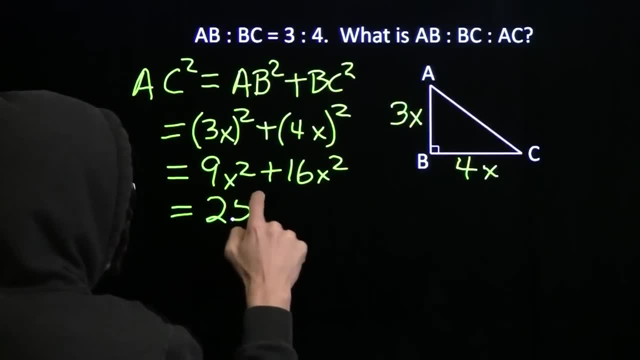 square the 3,, we square the x, We get 9x squared. Same thing over here. We'll get 16x squared. Add those up And we'll get 25x squared, equals AC squared. Now we know what we square In order to get. 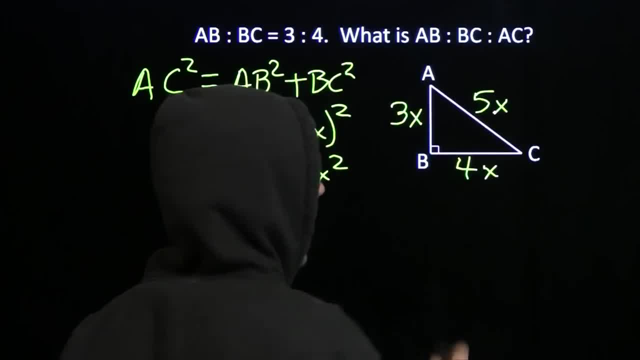 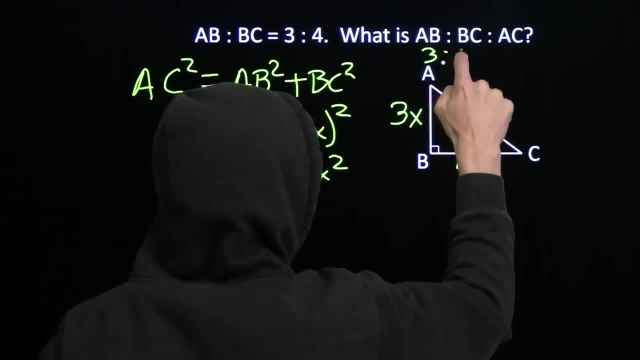 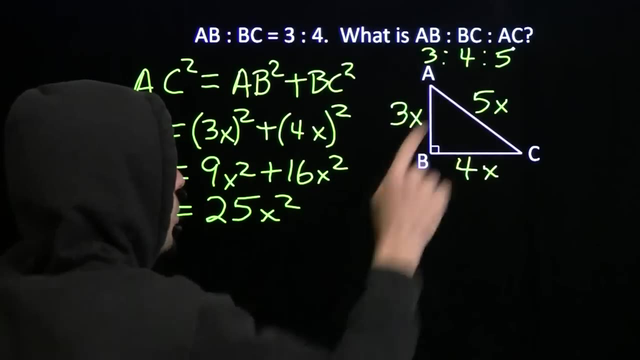 25x squared, we square 5x. So sure enough, this ratio of the three sides here is 3 to 4 to 5.. 3 to 4 to 5.. We call that a 3-4-5 triangle- Not a very clever name, but it'll do. 3-4-5 triangle, What that really? 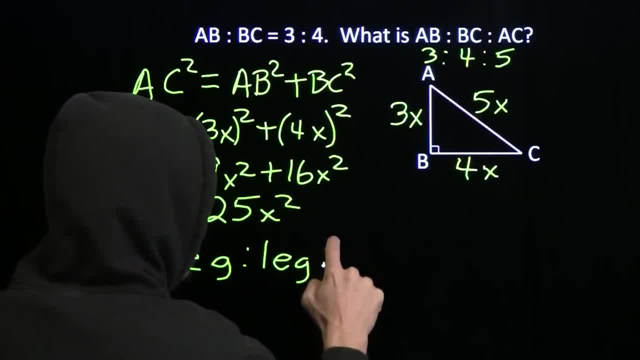 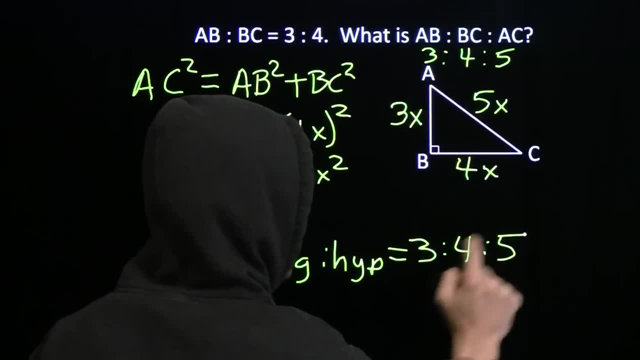 means is the leg to the other leg. Alright, so now we've got a right triangle. Now we're going to find the ratio of all three sides. So if we divide the leg to the hypotenuse, that ratio is 3 to 4 to 5.. Now this is really. 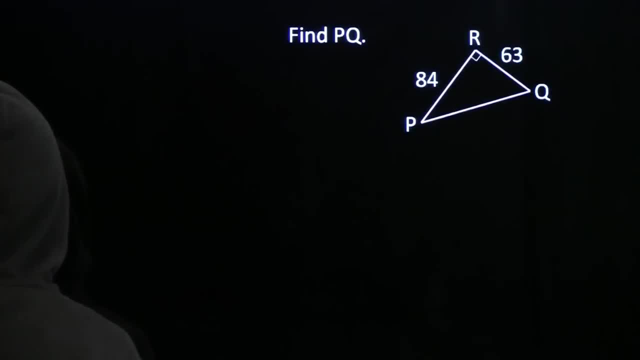 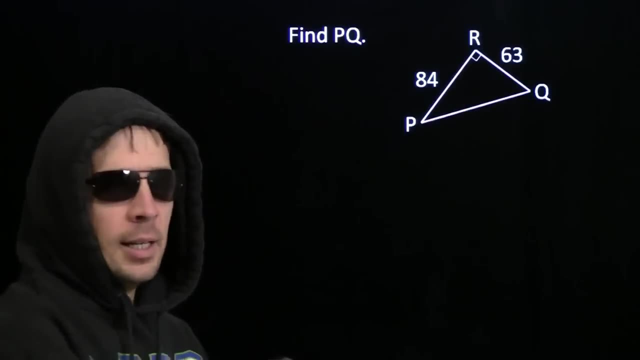 powerful. This is really useful stuff. Check this out. I'm going to knock off a few problems with this. Show you how powerful this is. We've got a right triangle here. We've got a right triangle. We've got two of the legs. Now maybe you see right off. I see right off. 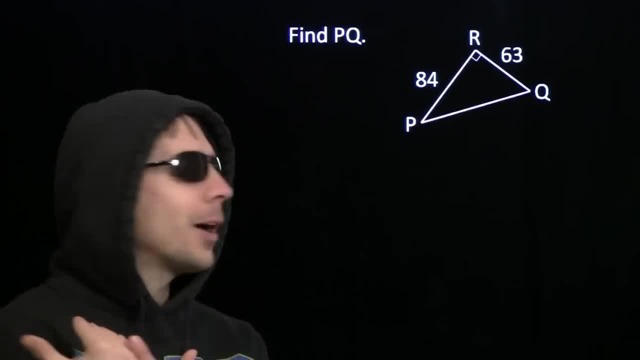 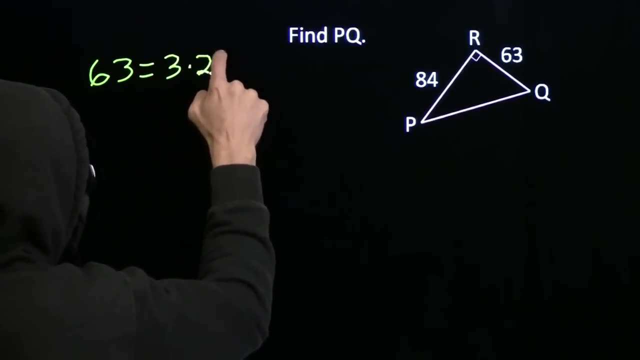 This is 3 to 4.. Of course it's going to be 3 to 4, because that's what we were just talking about. This is 3 times 21.. 63. 63. 63 is 3 times 21.. 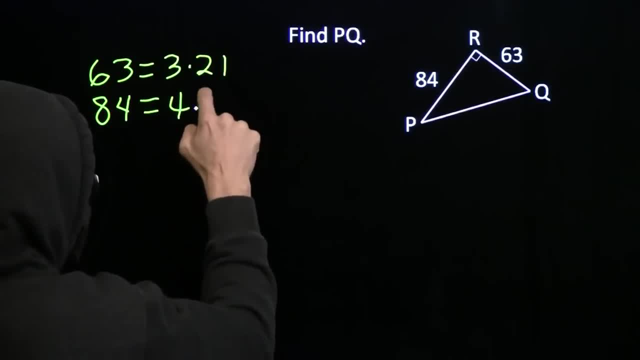 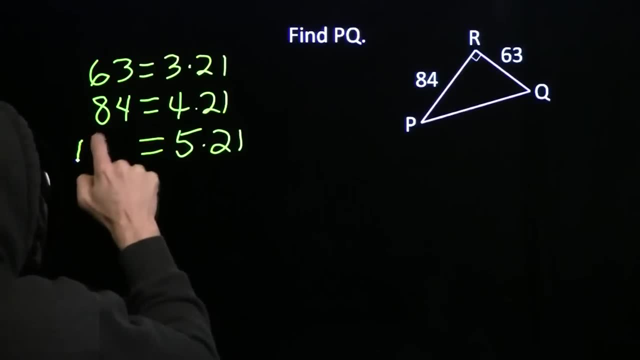 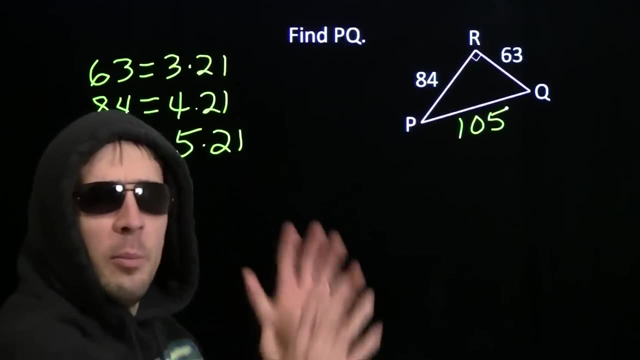 84 is 4 times 21.. So we know what the hypotenuse is going to be. It's going to be 5 times 21.. That's 105.. Now maybe you didn't see right away that this was 3 to 4.. Imagine we gave you this problem. 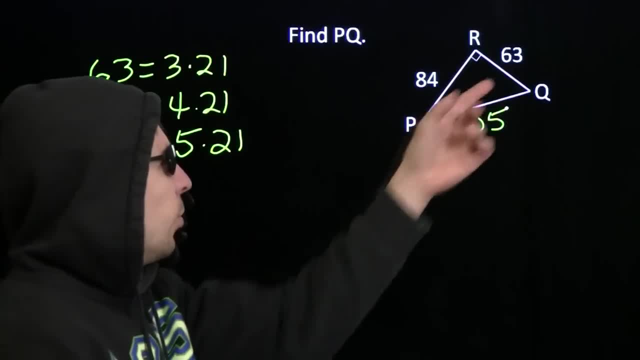 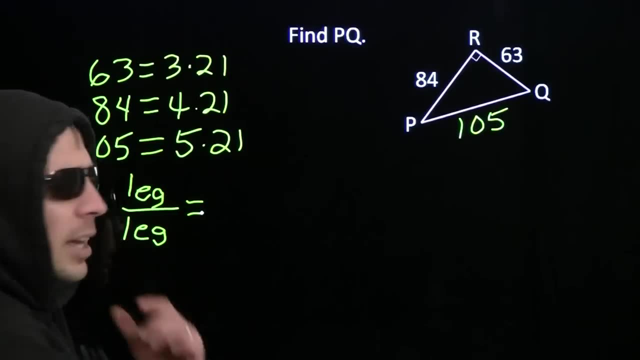 and hadn't just talked all about that 3-4-5 stuff. Well, I'd look at this and I'd say, okay, what's the ratio of one leg to the other? Because I'm given the two legs here, Leg to. 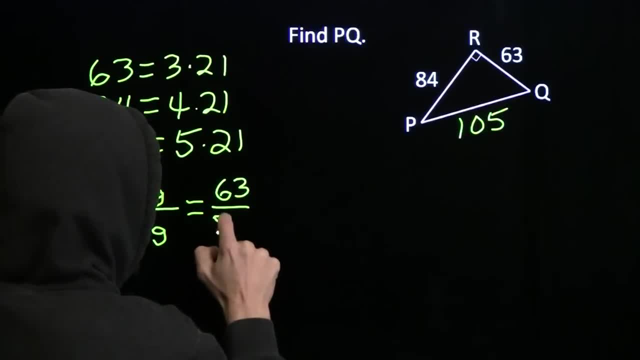 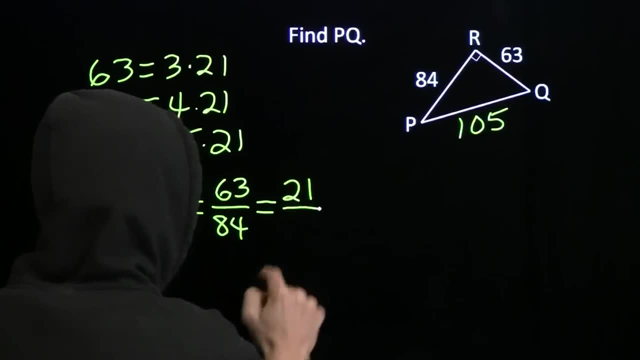 leg. my ratio is 63 to 84.. And then we'd simplify this fraction. We'd pull out common factors. You can pull out a common factor of 3. That'll give me 21 over 28.. And now I'll pull out. 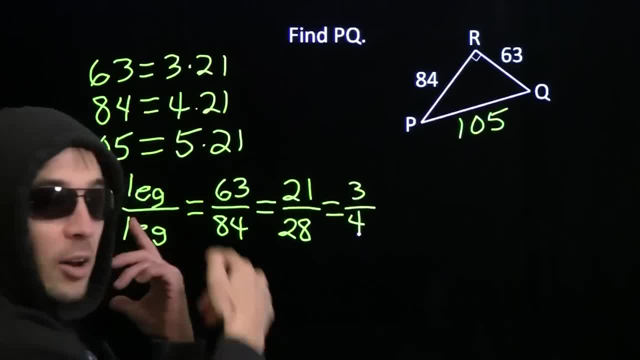 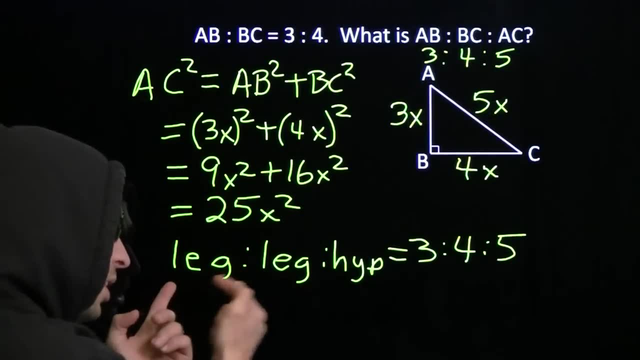 a common factor of 7.. And sure enough, aha. The ratio of leg to leg is 3 to 4.. Let's look back here: Leg to leg: 3 to 4.. That means it's going to be leg-leg Hypotenuse is going to be 3-4-5.. That's what we just 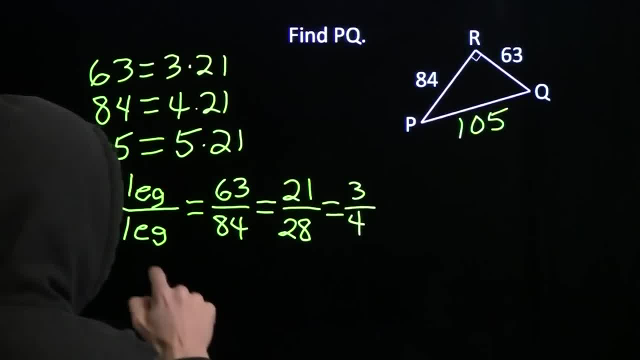 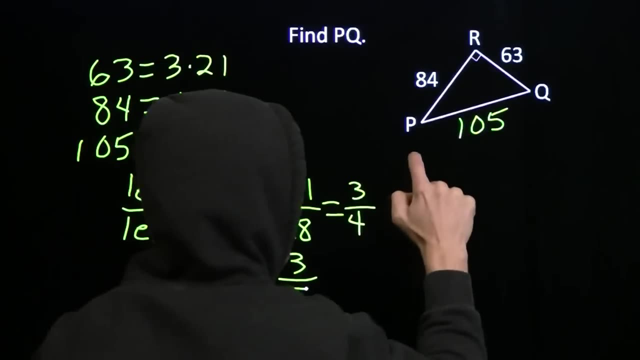 showed here. So I come back here and I know that, say, the short leg to the hypotenuse is going to be 3 fifths. Once I see the 3 to 4, I know I've got 3-4-5 triangle, I've 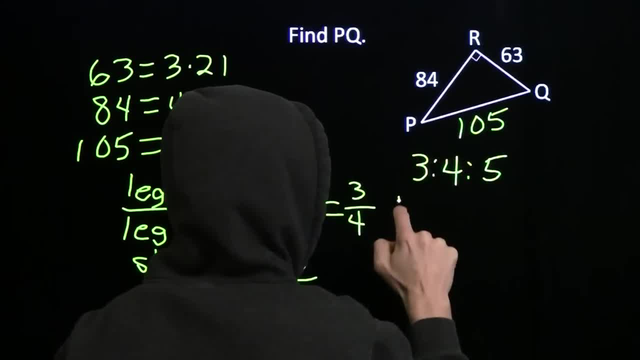 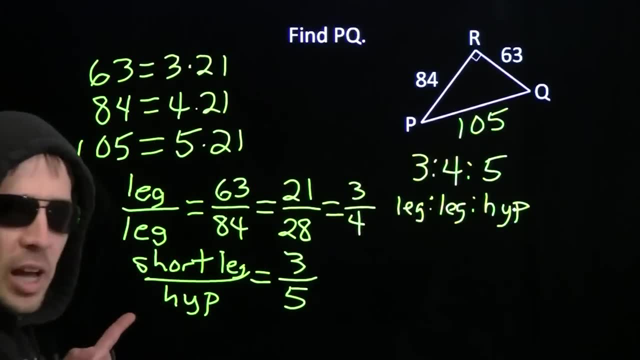 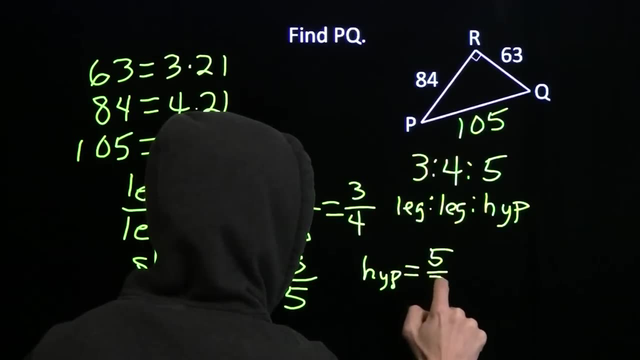 got 3 to 4 to 5 is the leg to the leg to the hypotenuse. So the short leg to the hypotenuse is 3 to 5.. That means the hypotenuse is 5 thirds times the short leg. 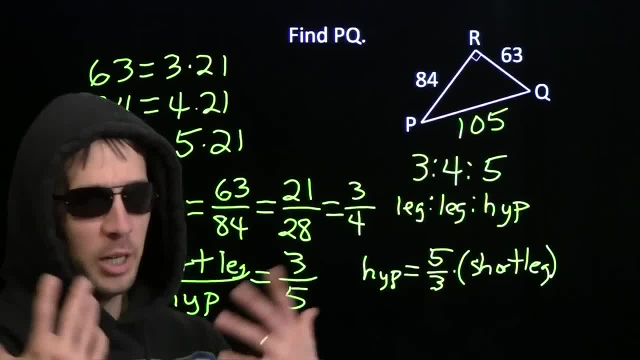 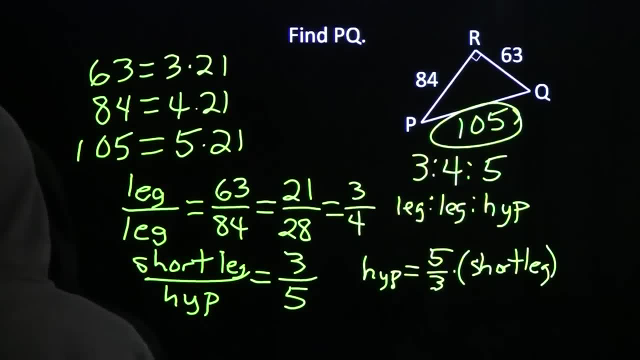 Now I just take my short leg 63, stick it in here. 63 divided by 3 is 21, multiplied by 5, and I get my 105 back. Let's try one more. Make sure we have this down. Whew, I'm. 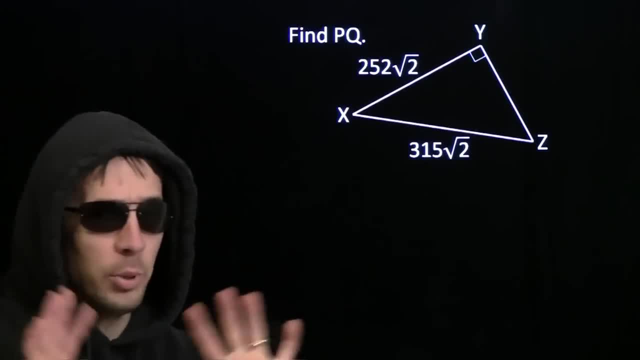 going to try this again. Now you take a look at this. Now you certainly don't want to break out the Pythagorean Theorem on this, because you want to square that, Have fun. So instead, we don't want to use. 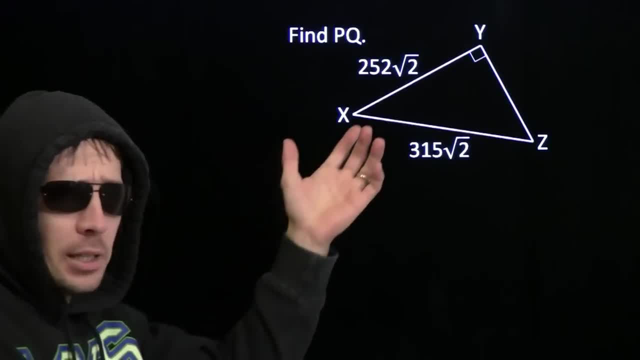 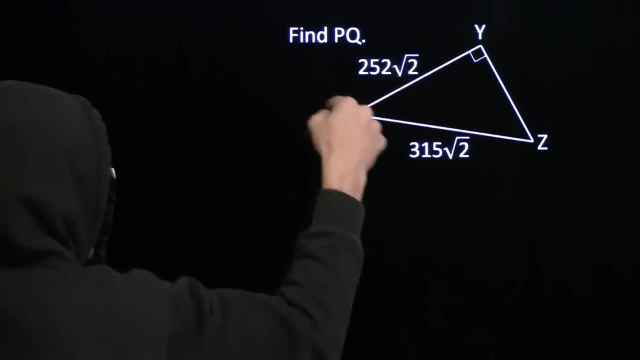 the Pythagorean Theorem. We want to do something clever, Not immediately obvious. This is a 3-4-5 triangle, But once again we'll go ahead and set up our ratios. Now we've got a leg and a hypotenuse, So we've got leg to hypotenuse is 252 root 2.. And then 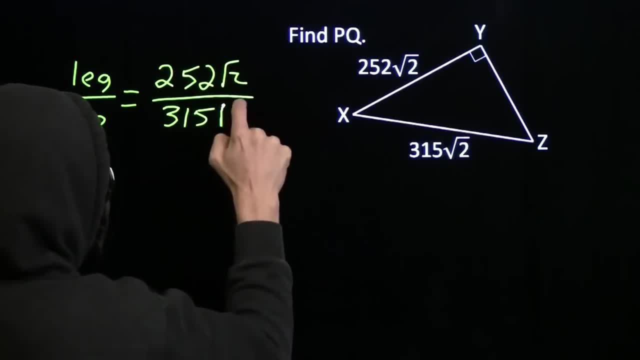 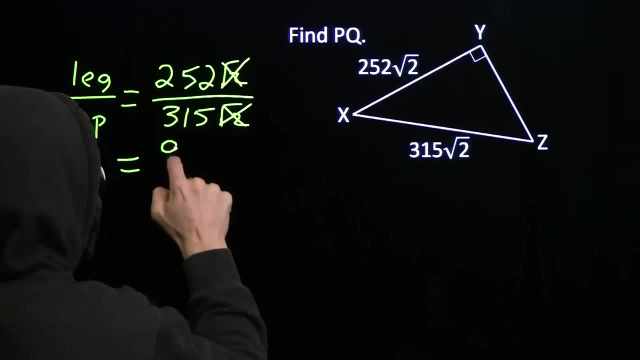 we've got a leg over 315 root 2.. Now we can cancel out the square root of 2.. And we're going to simplify this fraction. First we'll pull out a factor of 9.. 2 plus 5 plus 2 is: 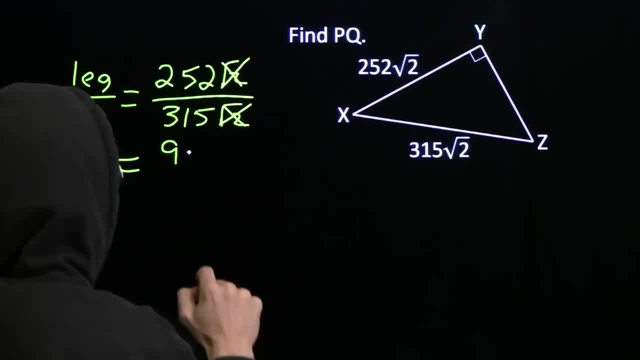 9.. 3 plus 1 plus 5 is 9.. These are both multiples of 9.. And I'll get 9 times 28.. And pull out a 9 here as well, It's 9 times 35. The 9s cancel 28 over 35. We recognize that especially. 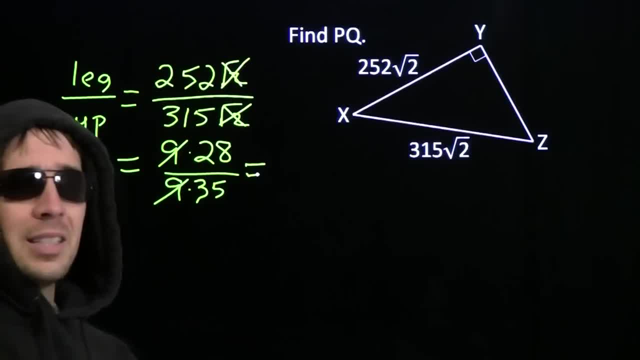 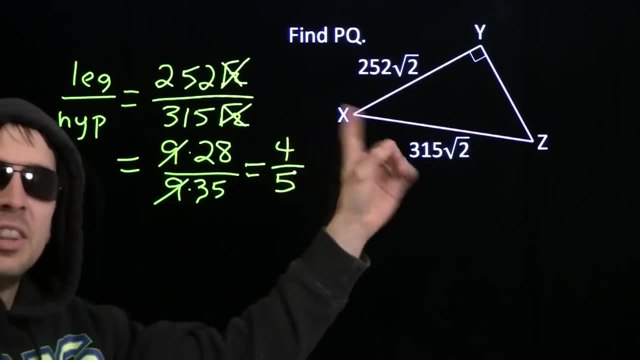 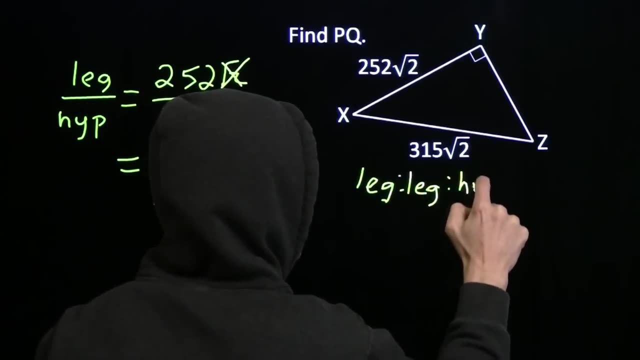 you football fans, 4 touchdowns over 5.. After 5 touchdowns you pull out the 7s, You're left with 4 fifths. Leg to hypotenuse is 4 to 5.. This is a 3-4-5 triangle, Again, leg to leg to hypotenuse 3 to 4 to 5.. And I've 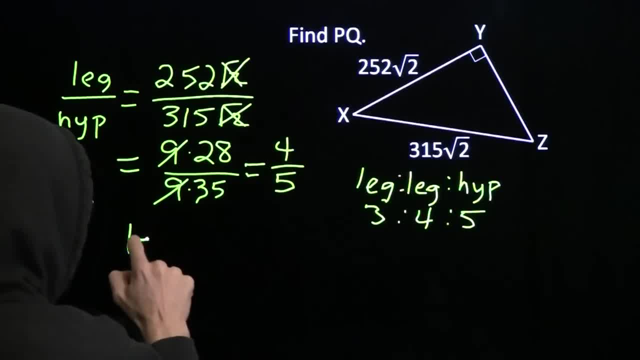 got leg to hypotenuse is 4 to 5.. So I know that the ratio of my legs is 3 to 4. And I've found the one that goes here. I've found the longer leg, the one that goes with. 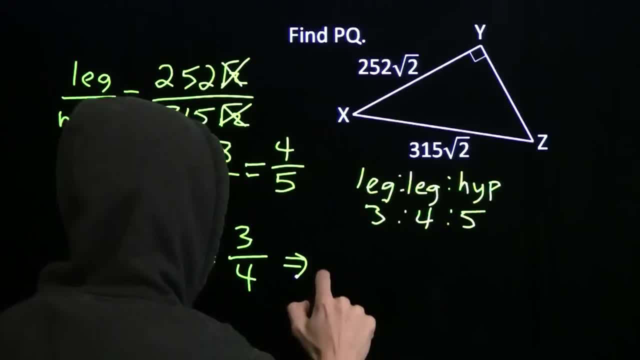 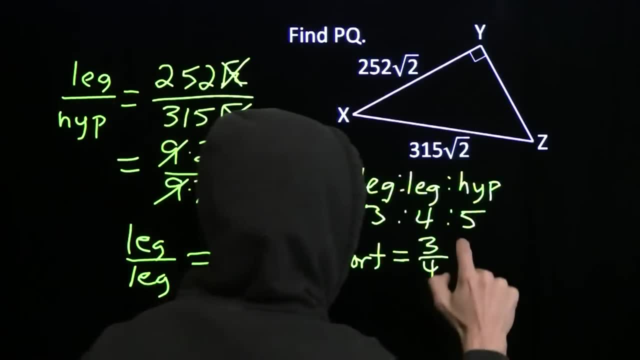 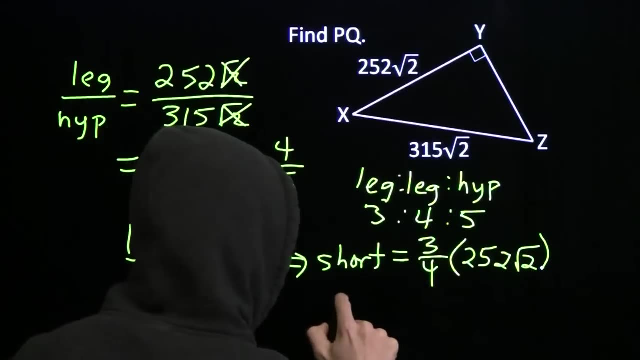 the 4 part of the 3-4-5.. So my short leg, the short leg is 3 quarters the long leg. So now I'm just going to divide 4 into 300, into 252 here And I'm going to have 3 times. 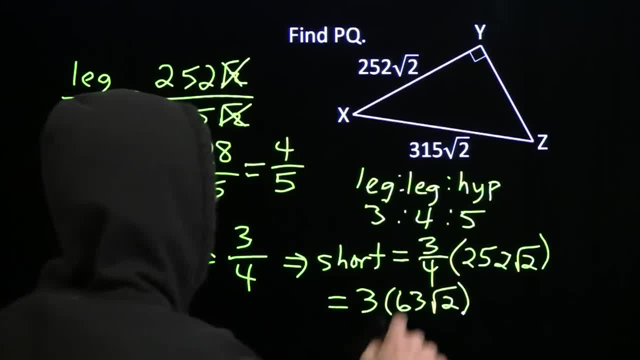 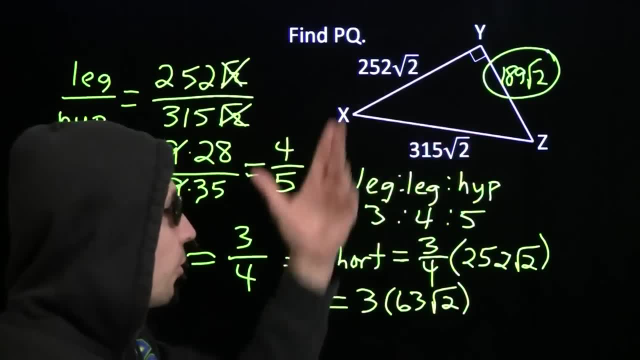 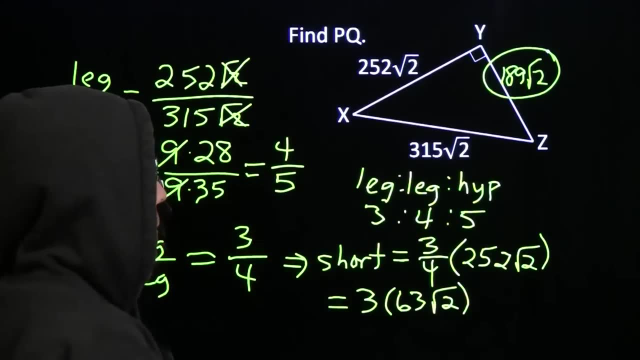 63.. Root 2. 3 times 63.. That's 189.. Root 2. Another 3-4-5 triangle And we solve the problem just like that, without ever breaking out the Pythagorean Theorem to square these really tough to square. 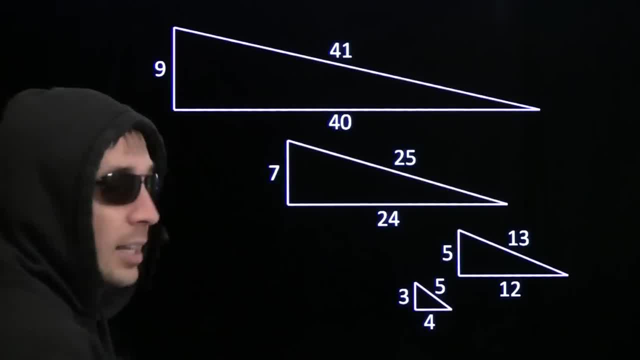 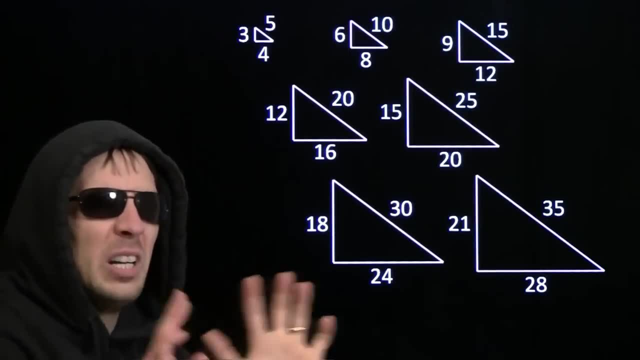 numbers. All right, I'm going to finish up by saying, hey, that first set, this first set here of triangles. these aren't the only triangles in the world. 3-4-5 are not the only triangles in the world. 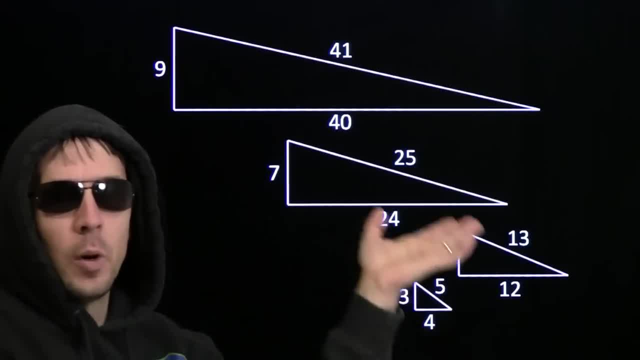 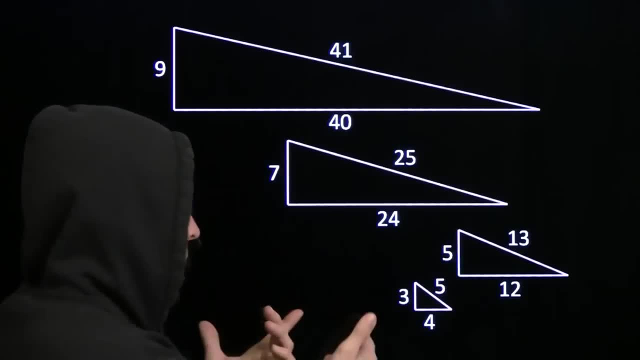 They're the only triangles in the world with integer side lengths. There are lots and lots more. Now here's a few I've found. We call, say, a set of three numbers that satisfies the Pythagorean Theorem. we call that a Pythagorean triple. 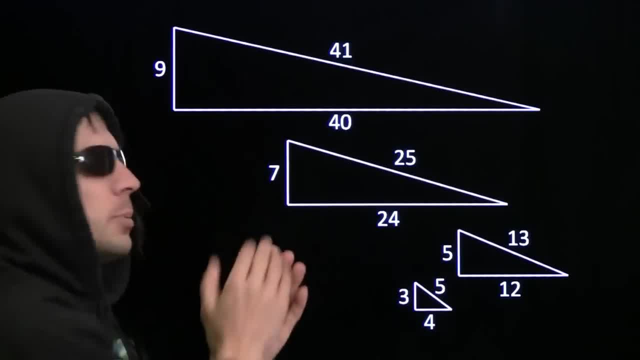 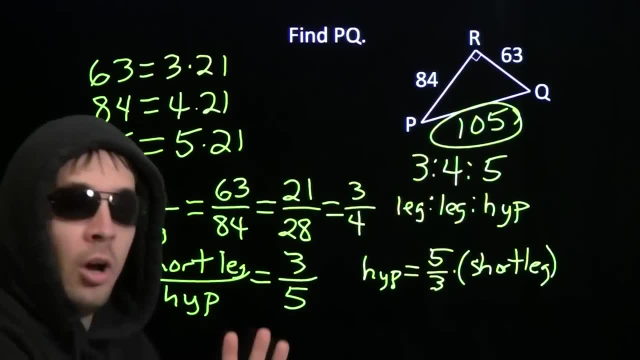 Now here are a bunch more of them, And we'd like to know these pretty well, because then we can do slick things like this, Because this isn't just good for 3-4-5 triangles, We can do this with all sorts of sets of Pythagorean triples that we know Now. these are very special. 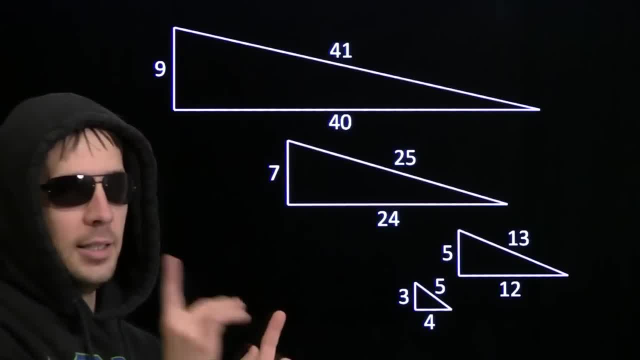 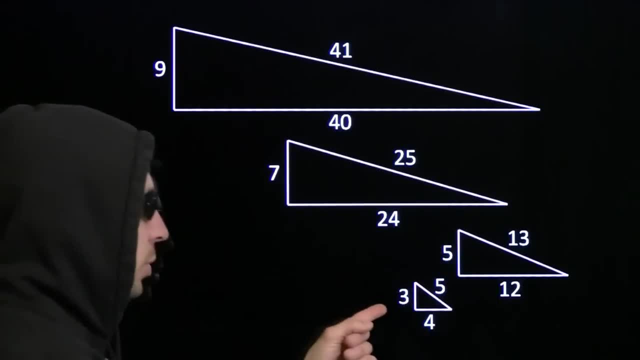 Pythagorean triples. There's a really cool pattern hiding in these. I'll explain the pattern, but you've got to figure out why it works Now. first the short legs. here they're the odd integers 3,, 5,, 7,, 9.. And the other the 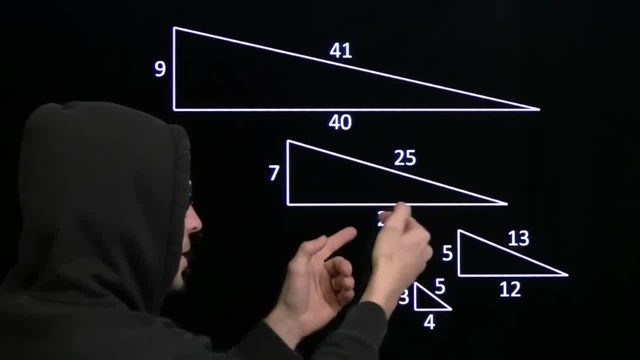 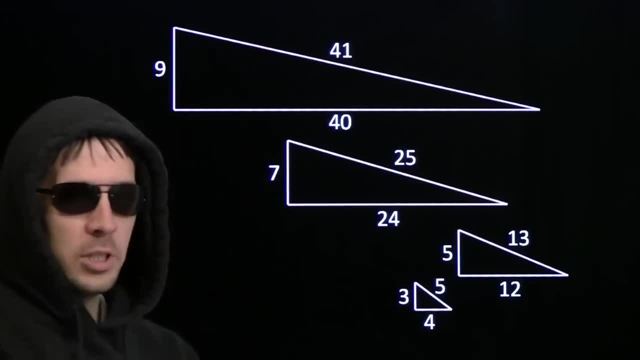 other sides. well, you'll see they're consecutive integers: 4-5,, 12-13,, 24-25,, 40-41.. Now here's where it gets really cool: 4 plus 5 is 9.. That's 3 squared. 12 plus 13 is 25.. That's.